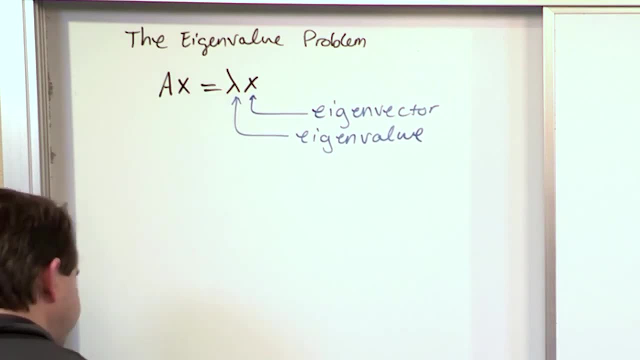 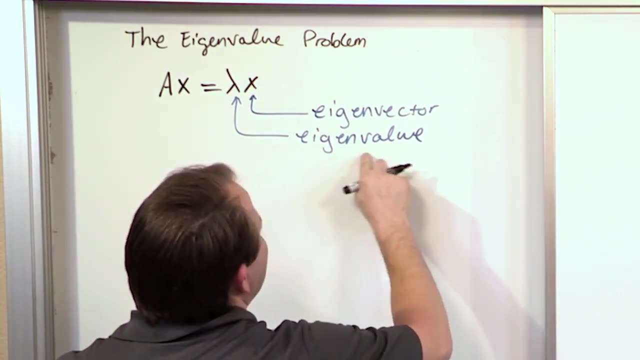 direction of symmetry in objects. So that's just one example, but I think it's good to have some grounding. Let's take a little bit of a closer look at this. The eigenvalues, these are just scalars, Right? And so the eigenvalues, these are just scalars. And so the eigenvalues, these are just scalars. 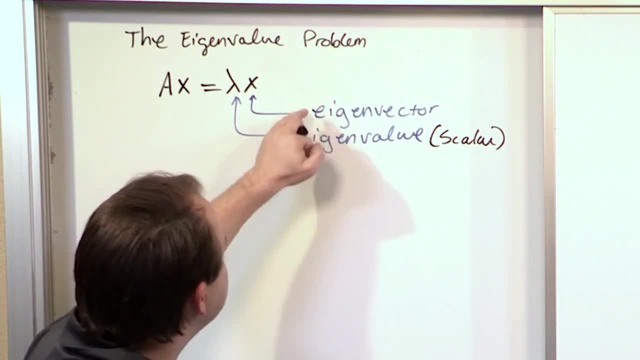 The eigenvector. I'm not going to write it there, but it's a vector. The word eigen is just a German prefix. Don't worry so much about what that means, but basically these are special vectors associated with this matrix and special values associated with this matrix. What do you think makes them? 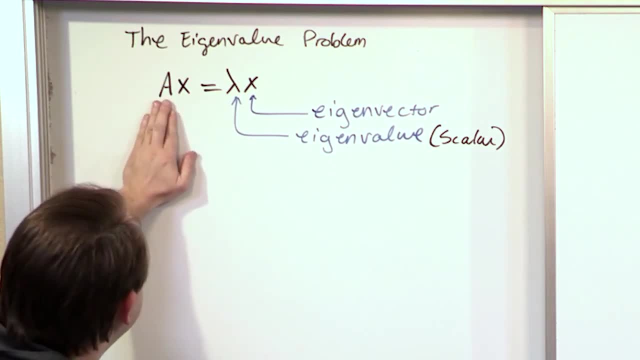 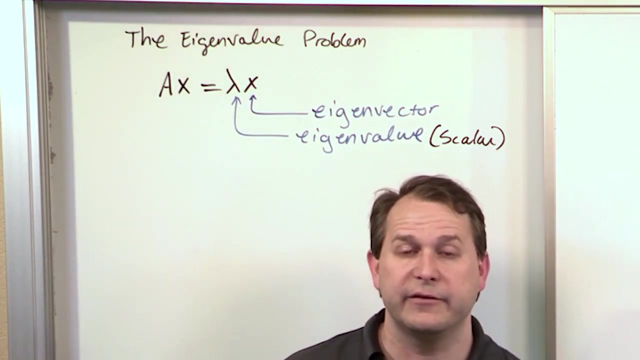 special. What it's basically saying is if I take the matrix A and I multiply it by an eigenvector, X okay, then when I get on the right-hand side is the same eigenvector but multiplied by a scalar. So it's a special solution of the matrix where when you put that vector into the left-hand side of the 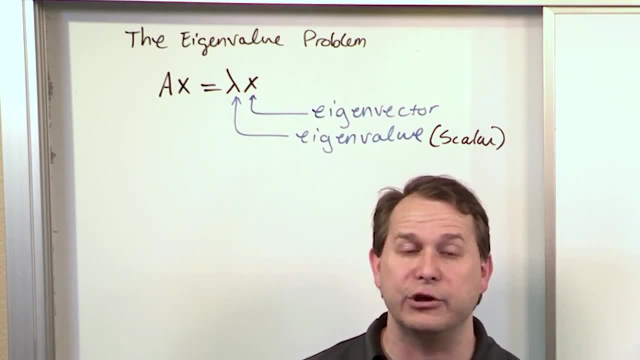 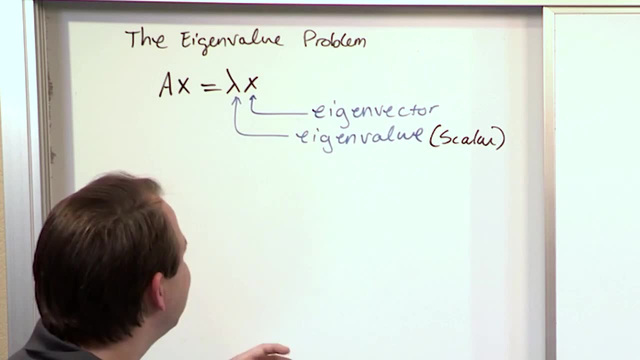 equation, you get the same vector back, but just scaled by a value, the value that we call the eigenvalue. All right, That's why it's called eigenvalues and eigenvectors. So make sure you understand that, Just conceptually, what it is is a special solution of this equation, such that when, if you stick it, 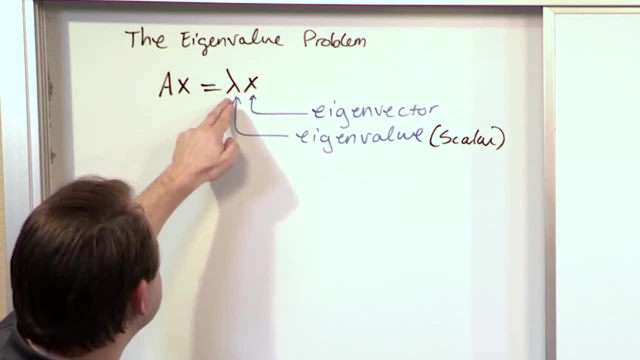 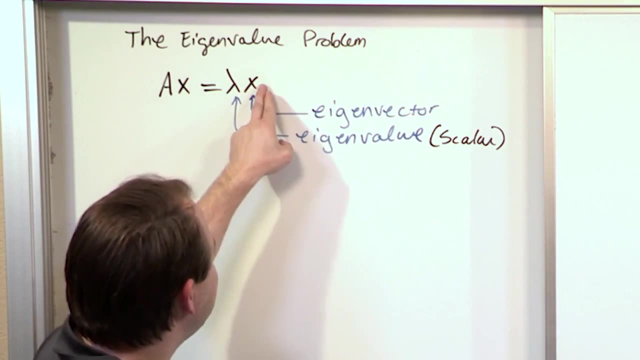 back in the left, you get the same thing out, but scaled times a constant. And remember, these are vectors. They point in the same direction. right, X and X point in the same direction And even if you take X and multiply it by a number, 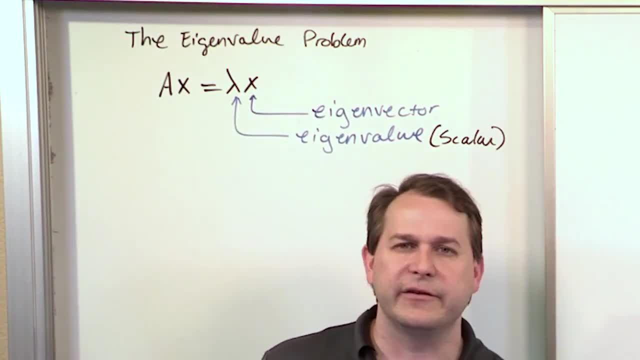 it's still going to point in the same direction. So what it is is a vector that points in a certain direction. You stick it in the left, you get back another vector that points in the same direction, but it's scaled, which means it's maybe longer or shorter. okay, For every eigenvalue lambda, there is a set of non-trivial vectors, X. 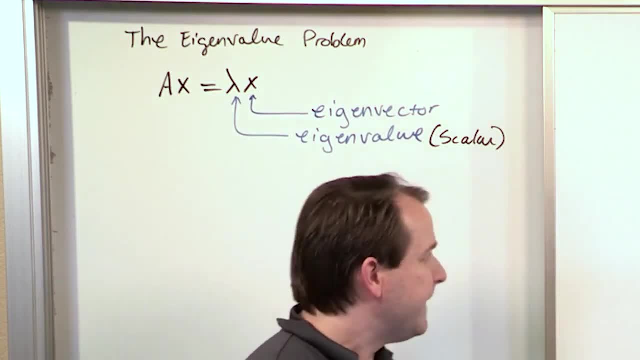 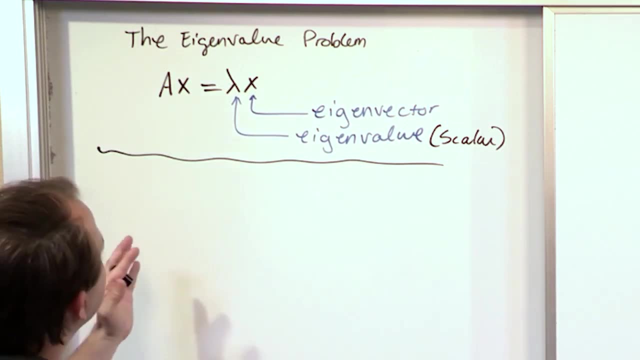 that we call eigenvectors. I want to say that out loud because I have it written on my paper. So, now that you have the general idea of what the eigenvalue problem is, ultimately, what we're going to figure out how to do soon is how to calculate these eigenvalues and how to calculate the corresponding eigenvectors. 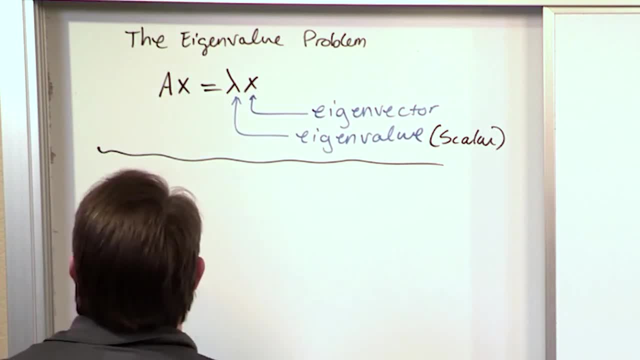 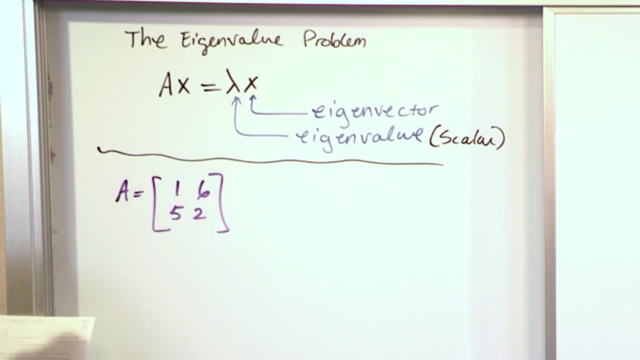 But before we get to that, we're going to do a simpler problem. I'm going to give you a matrix A, in this case 1, 6,, 5,, 2.. And I'm going to give you a vector X1, 6, negative 5.. And I'm going to ask you: 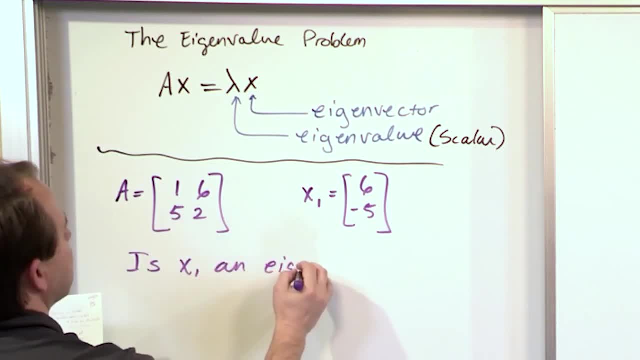 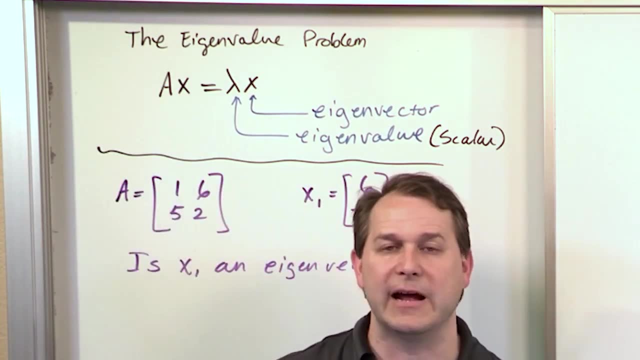 is X1 an eigen 1, 2, 1, 1, 2, 1, 2, 1, 2.. So ultimately, you need to be able to have a matrix and calculate the eigenvectors. 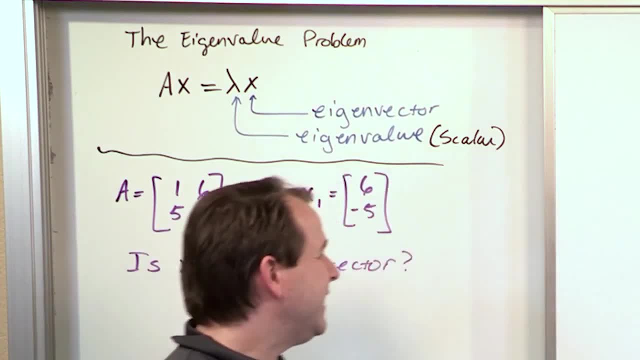 and eigenvalues. We're not doing that yet. We're going to take baby steps. I'm gonna give you a matrix and I'm gonna ask you: is this an eigenvector of this matrix? And you have to answer yes or no. 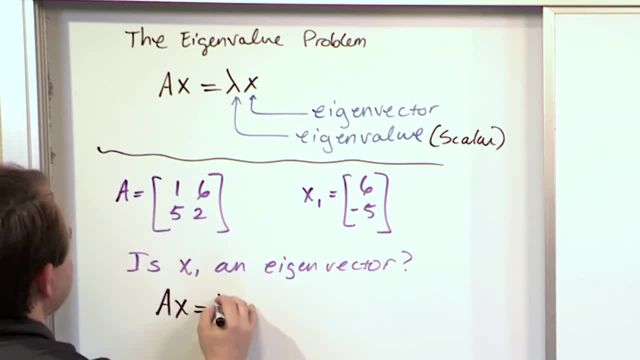 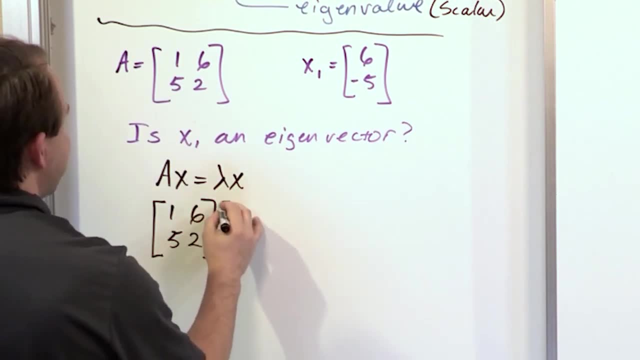 Well, the way to figure it out is: you go back to your definition. AX is lambda X, So let's stick it on the left hand side. A is 1, 6, 5, 2.. And the test vector that we have—the 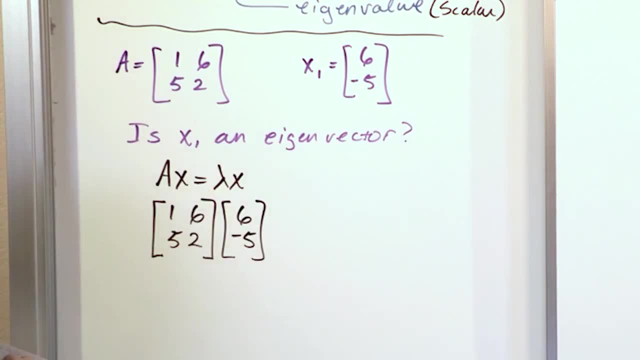 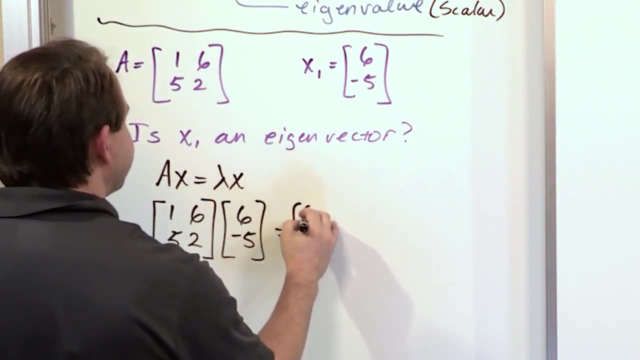 potential eigenvector is 6 times negative, or 6 and negative 5.. Now we need to do some matrix arithmetic here, so we're going to go over and down. okay, So 1 times 6 is 6,, 6 times 5 is negative. 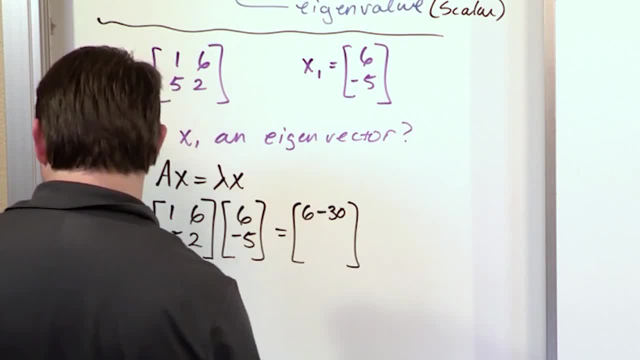 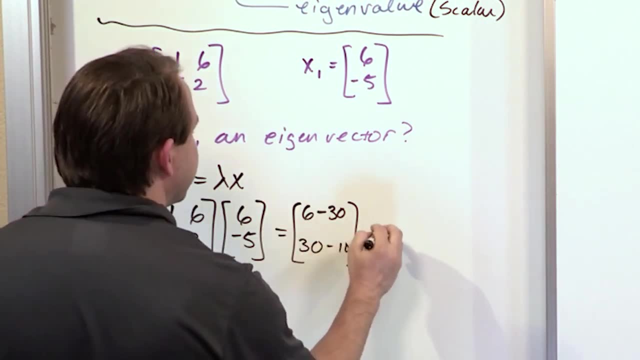 30, since it's negative 5, so I have negative 30 here And then going over and down, 5 times, 6 is 30, and 2 times negative 5 is negative 10.. So this matrix when I plug in the potential eigenvector. 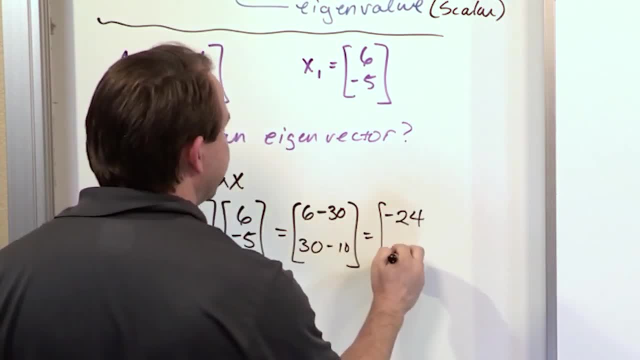 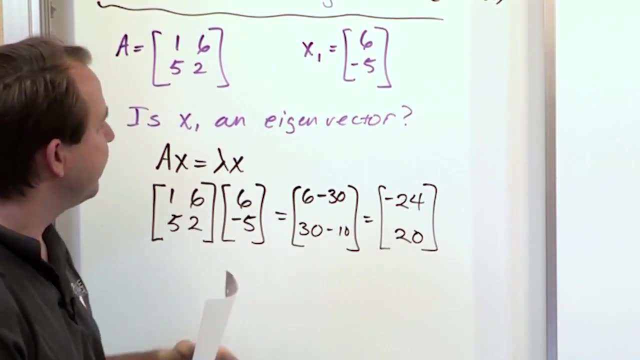 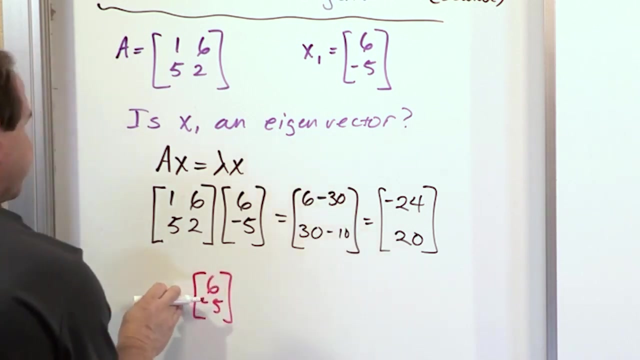 I get negative 24, and on the bottom I just get 20.. And the question is: is what I get when I plug this in the left-hand side? is it a multiple of the original vector? The question is, can I take this original vector, which is 6 and negative 5, and can I multiply it by something to give me? 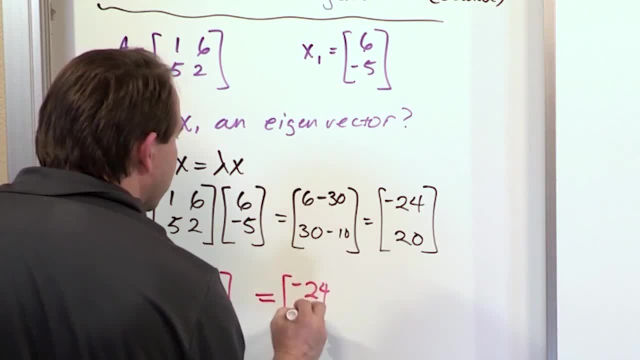 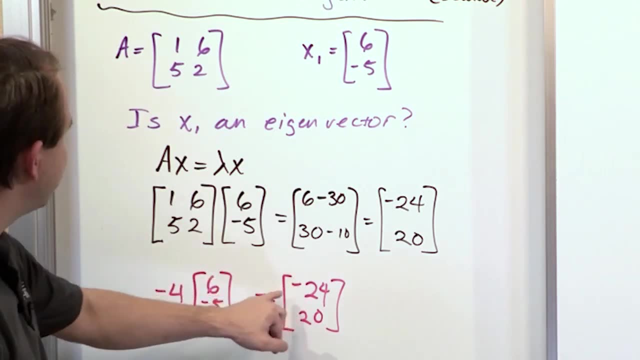 what I have just gotten on over here: negative 24 and 20? Is this possible? The answer is yes. What if I multiply by negative 4? Negative 4 times 6, is negative 24.. Negative 4 times negative 5 is positive 20.. Because there is a relationship here. 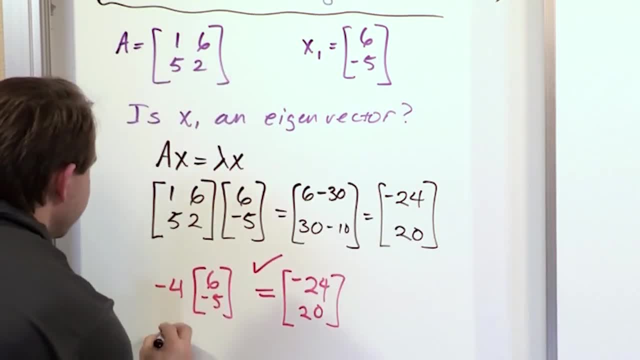 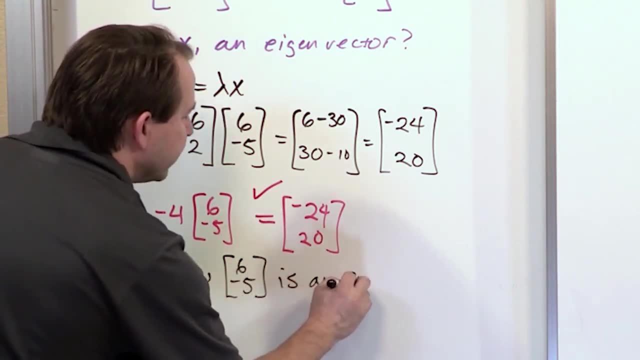 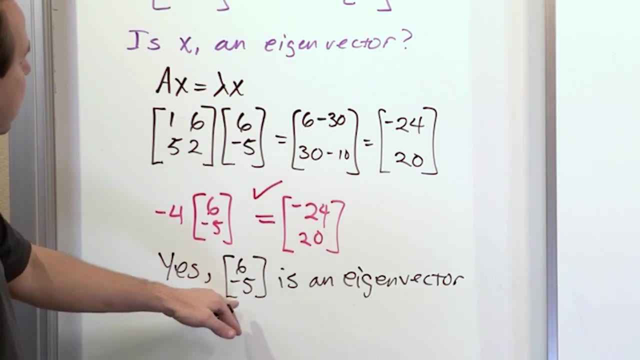 we can say actually two things as a result of this. Yes, 6, negative 5 is an eigenvector. Here's a bonus question for you: What is the eigenvalue that corresponds to this eigenvector? Well, lambda, which is the eigenvalue, is what sits in front. 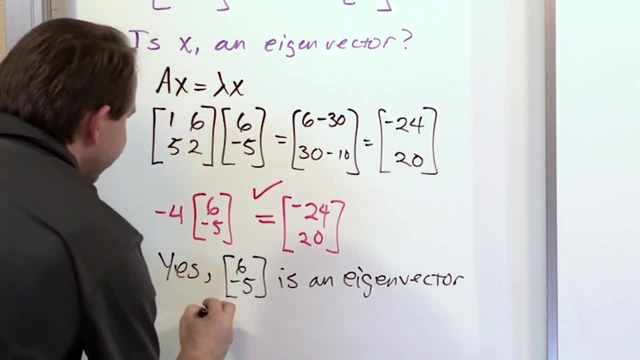 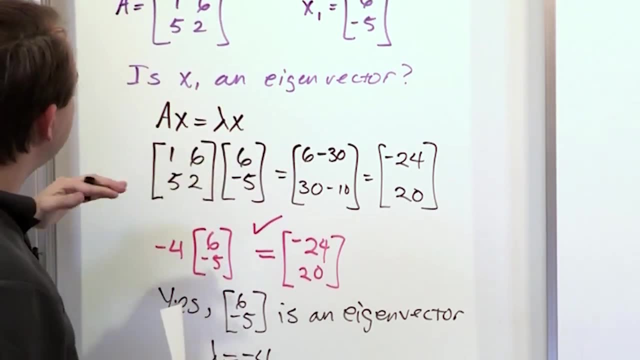 on the left hand, on the in front of the vector over here. So we say that in this case, lambda is negative 4.. Make sure you understand this. What we're saying is this is the eigenvector equation. In order for eigenvectors and values to be solutions, they have to satisfy the eigenvalue. 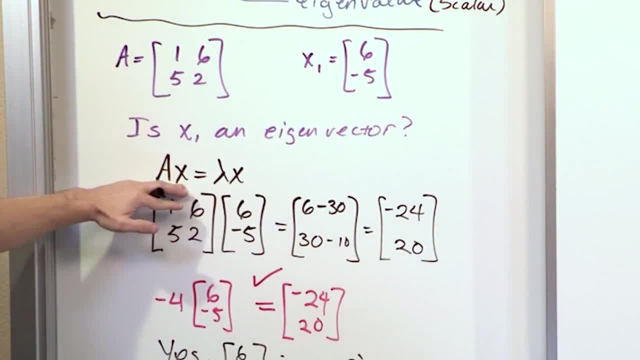 problem. So we take our potential eigenvector, we stick it in the left-hand side and we get this. And we have to ask ourselves: is what we calculated here a multiple of the original vector? And we find out that it is a multiple of the original vector. The multiple happens to be negative, 4. So 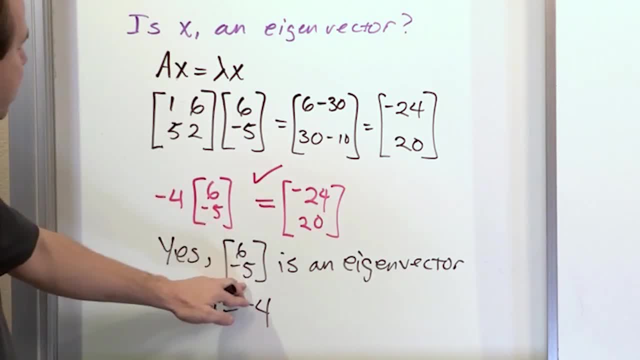 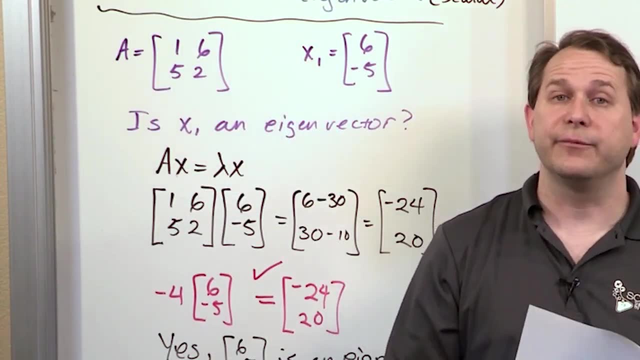 with the eigenvalue ends up being negative 4, the eigenvector ends up being this: All right, So again, we haven't gotten to the full glory of the problem. We haven't calculated the eigenvectors from scratch or the eigenvalues from scratch, But still these kinds of problems are really 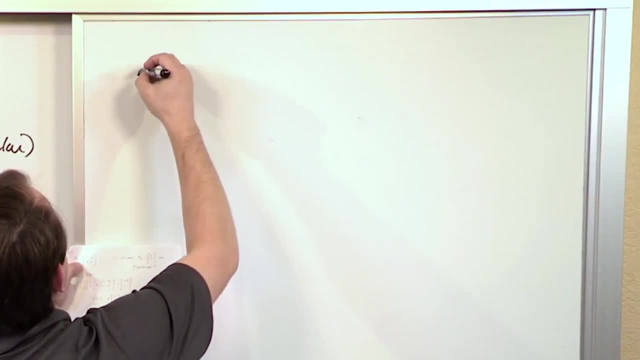 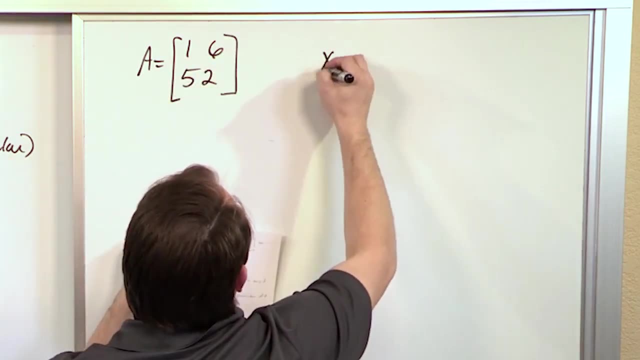 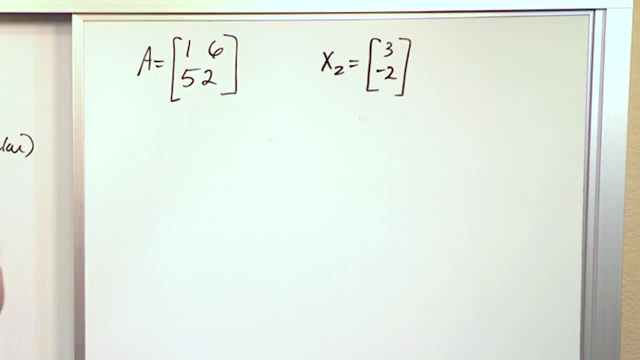 eigenvector of the problem or of this matrix. So we check it out. We say: well, is ax equal to lambda x? The matrix is 1,, 6,, 5, 2.. The test vector in question is 3 and. 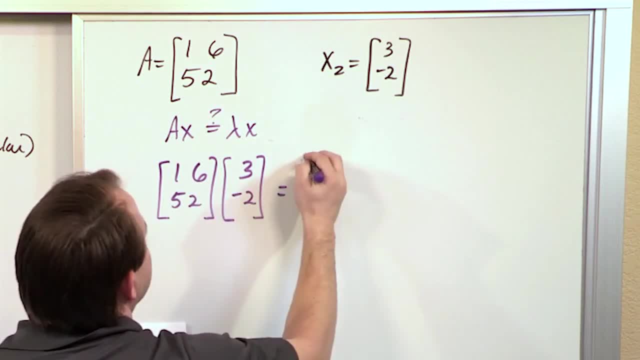 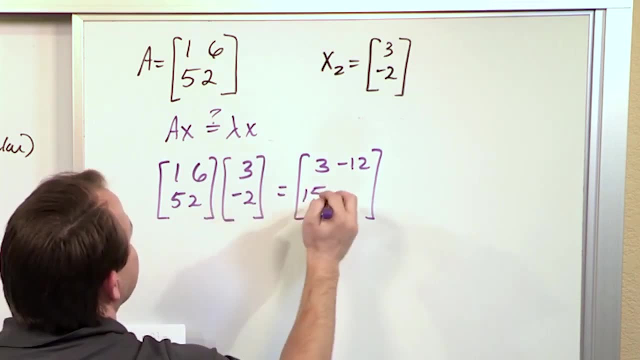 negative 2.. What do we get? 3 times 1 is 3.. 6 times 2 is negative 12.. 5 times 3 is 15.. 2 times negative 2 is negative 4.. So what I end up getting here? 3 minus. 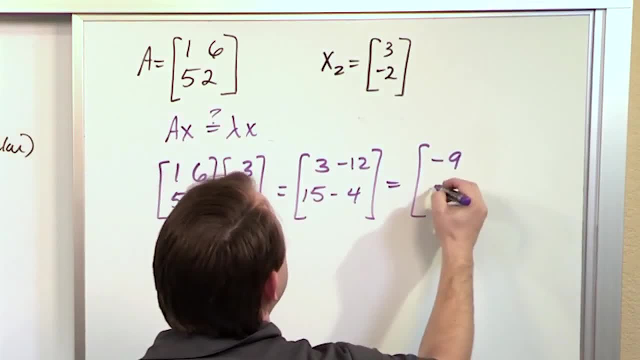 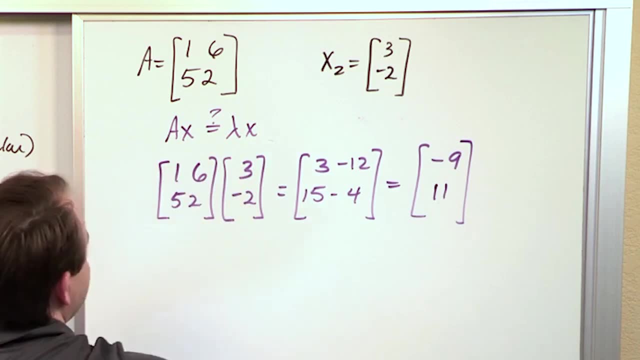 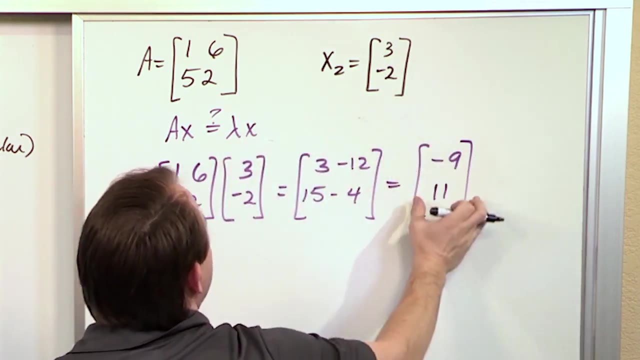 12 is negative 9, and 15 minus 4 is positive 11.. So what I end up getting is negative 9 and 11.. That's what happens when I plug this into the left-hand side. So the question is: can I find a multiple of this original vector that will? 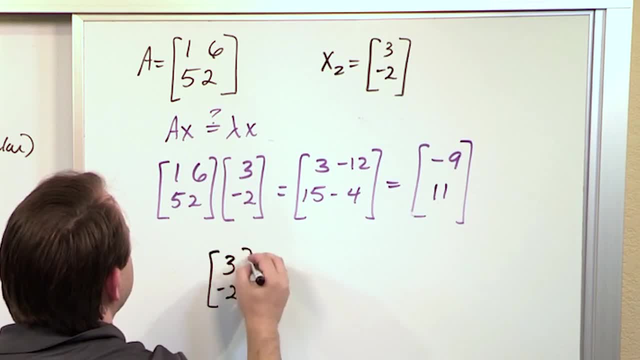 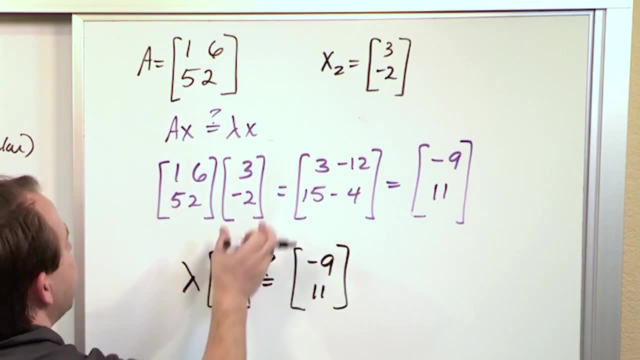 give me this. So the original vector is 3, negative 2, lambda times this. Can this be equal to negative 9 and 11?? Can I take a multiple of the original vector and have it equal what I've already calculated over there? Ask yourself that. Well, how do? 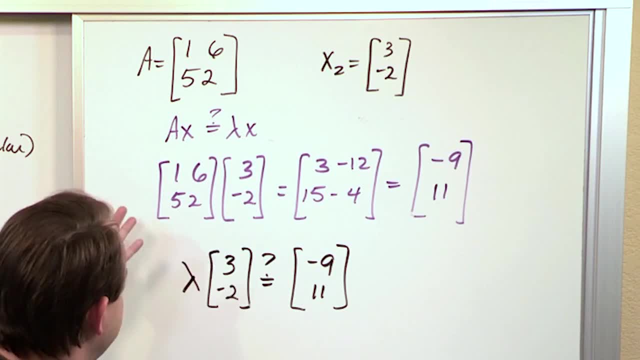 you get 3 to be negative 9? Well, you have to multiply by negative 3.. But if I multiply this by negative 3, there's no way it's going to be equal to 11.. There is no multiple that I can multiply my original vector by to give me what I 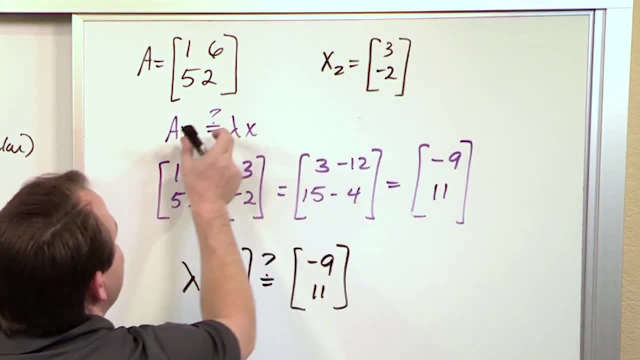 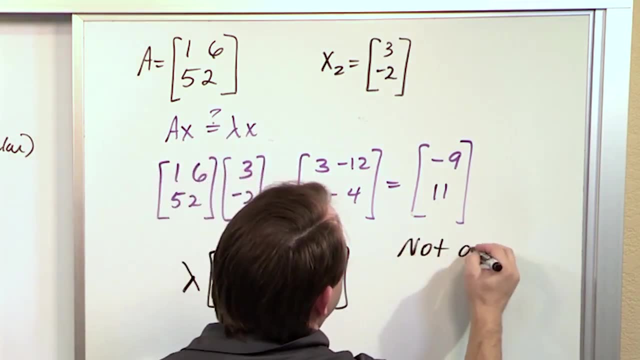 just calculated. So there's no way that this vector, when I put it in here, can be a scalar multiple of itself when I run it through this matrix. So not an eigenvector. So not an eigenvector. So not an eigenvector. 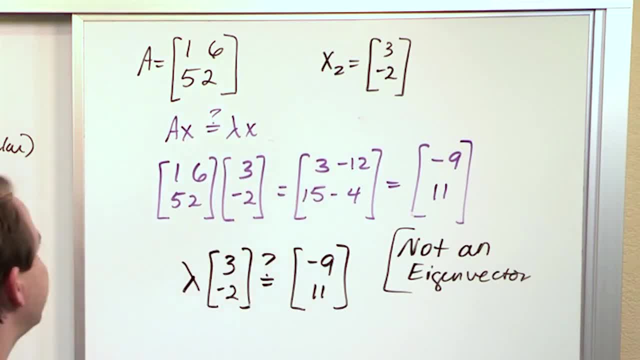 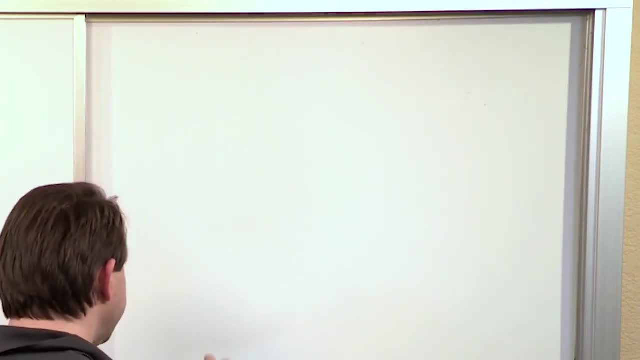 So there's no eigenvalue associated with it. There's no eigenvector. There's nothing special about this guy. This is just another vector. It's a test we ran. Failed the test with flying colors. Now, those were 2 by 2 matrices, but the exact same thing holds for 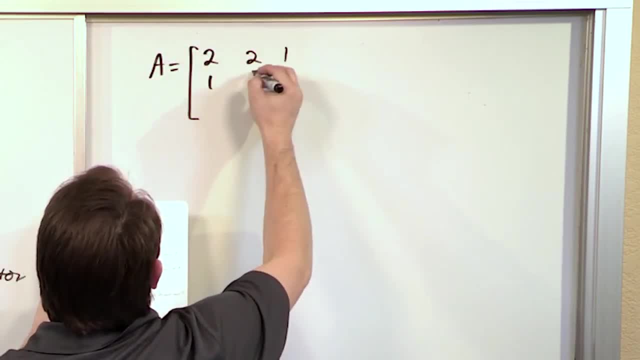 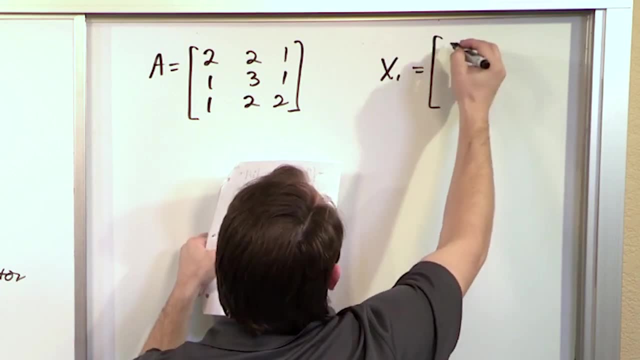 larger matrices. What if I have 2, 2, 1, 1, 3,, 1, 1,, 2, 2, and I want to test this vector and see if it's an eigenvector- Negative 1,, 1,, 3.. 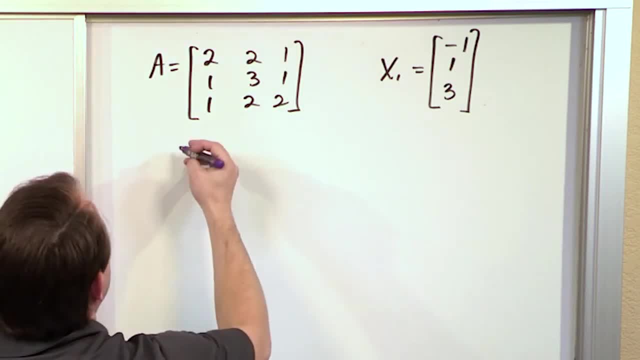 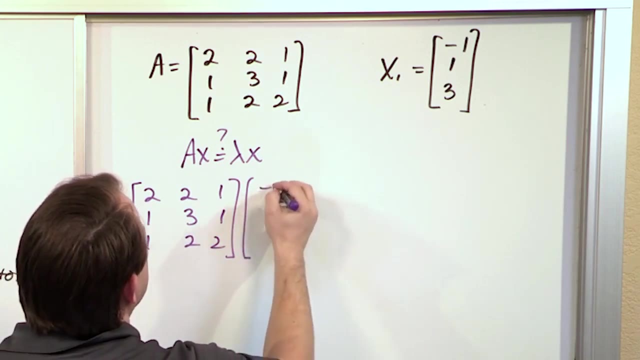 Okay. so how do I do it? Well, I've got to run it through the eigenvalue or the eigenvector equation. Ax is lambda x. I'll have to test that for equality. So when I put it in here: 2, 2, 1,, 1,, 3,, 1,, 1,, 2,, 2, and I just write down the matrix negative: 1, 1,, 3,, let's do. 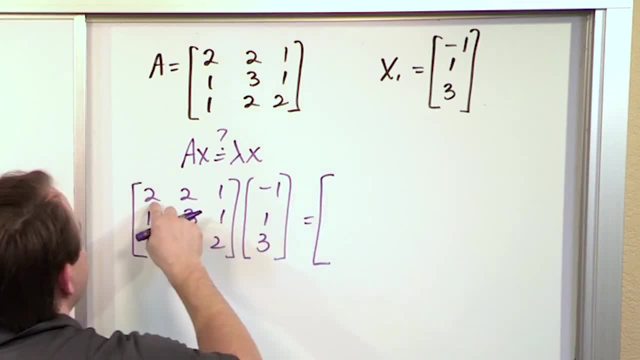 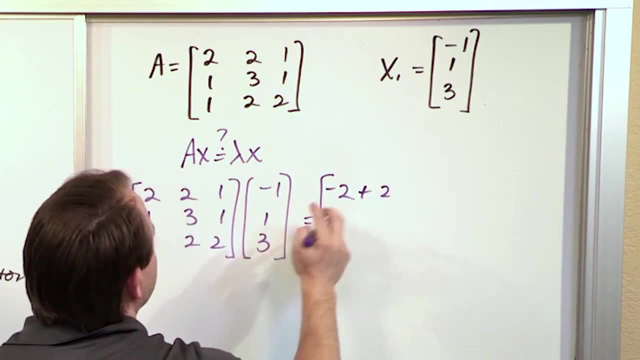 this multiplication here. So what I will have is 2 times negative. 1 is negative, 2, 2,. I'm going to go down like this: 1 is 2.. 1 times 3 is 3.. I go over and down here. This gives me a negative 1.. This times. 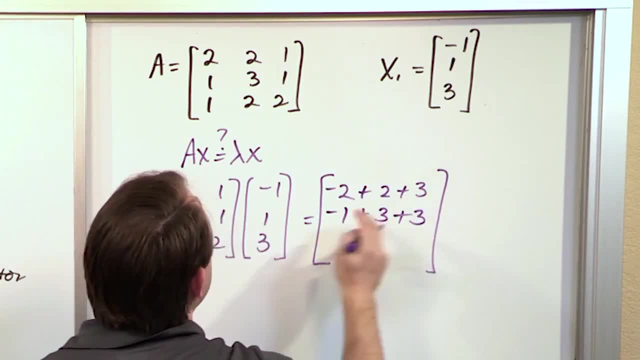 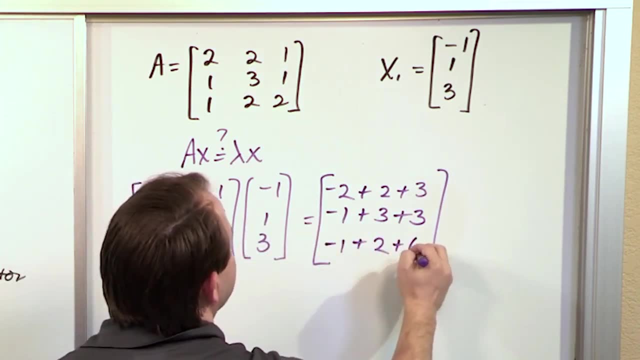 this gives me a 3.. This times this also gives me a 3.. And then I go over and down. This gives me a negative 1.. This gives me a 2. And this gives me a 6.. So when I run through, 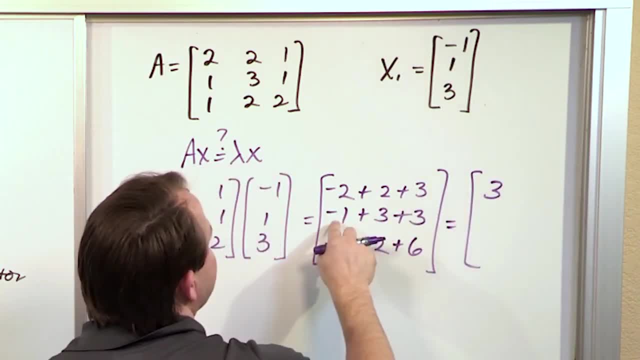 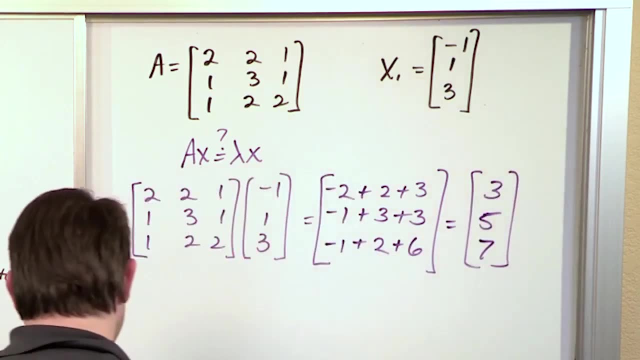 all of that, this goes away giving me only 3.. This is going to be a. 2 plus 3 is 5.. And then this is going to be: 1 plus 6 is 7.. So I get 357.. 357 there, And the question is: 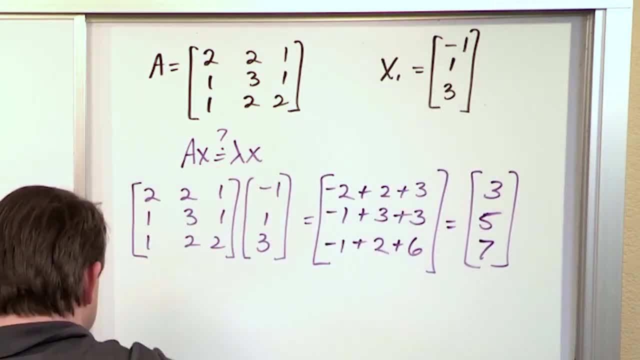 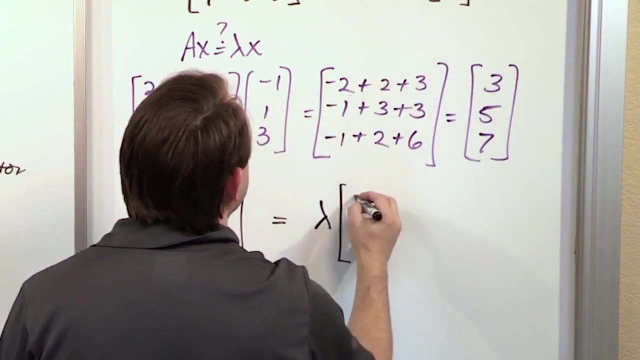 is this a scalar multiple of my original vector, Such that I can multiply it by an eigenvalue and get it So to formalize that? the question is: can I take 3,, 5, and 7 and write it as some kind of multiple of my original vector Negative 1,, 1,, 3.. Is there any way you can? 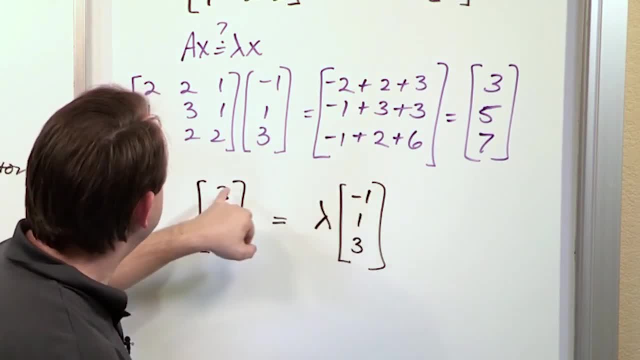 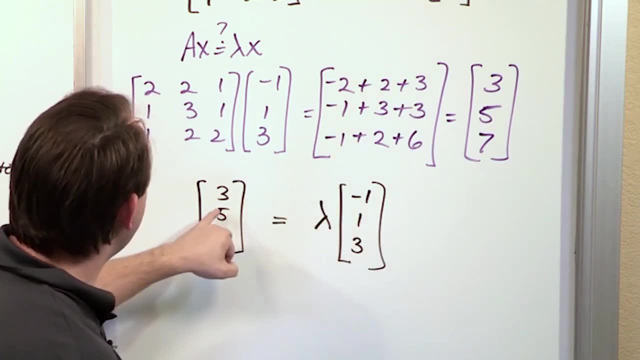 do that. Well, if I multiply this times to get 3, I'd have to multiply this by negative 3, right, Negative 3 times negative 1 to give me that. But if I multiply by negative 3, there's no. 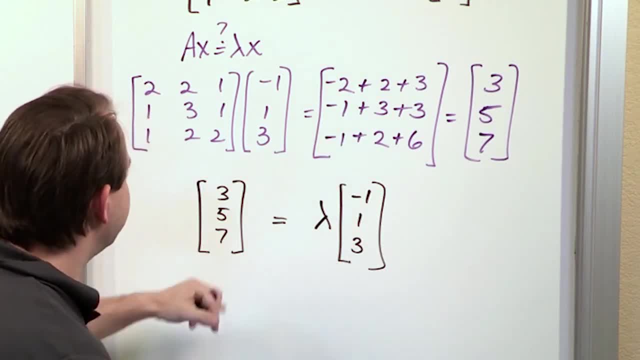 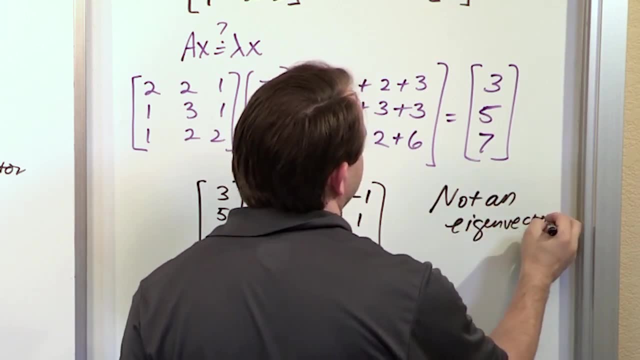 way I'm going to get that, And there's definitely no way, by multiplying by negative 3 that I'm going to get that. So this vector is not an eigenvector. All right, So you see the idea here. I want to do one more with you. These are really great little test questions, or? 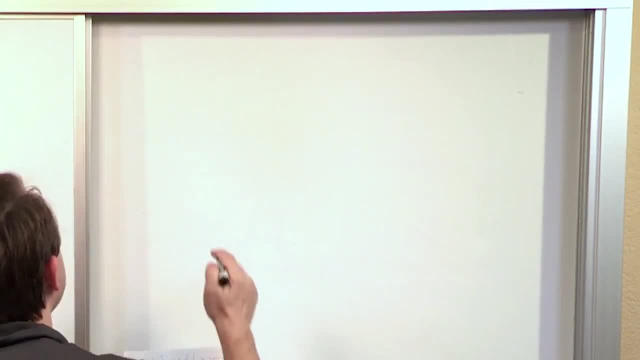 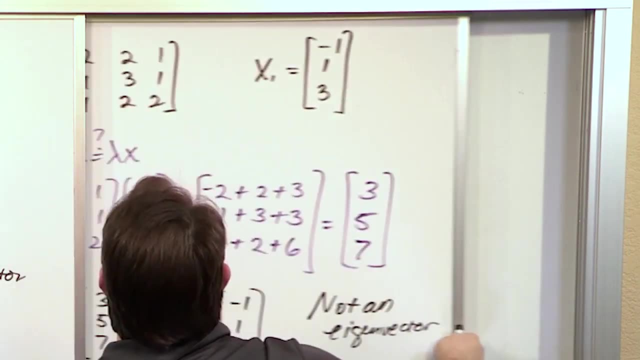 quiz questions, And I'll give you a little bit of a preview. This one will be an eigenvector. There's no way you can tell ahead of time until you run it through and test it. So 2,, 2, 1.. In fact, this is the same matrix. We're going to use the exact same matrix: 2, 2,. 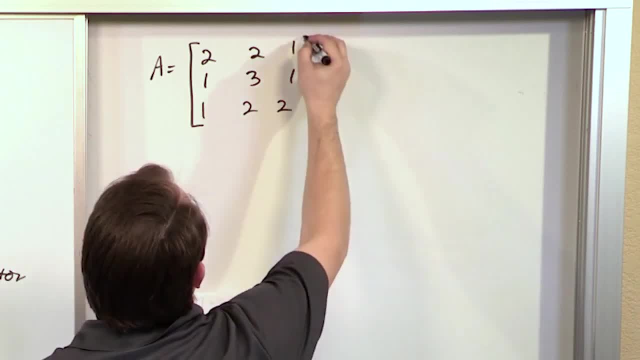 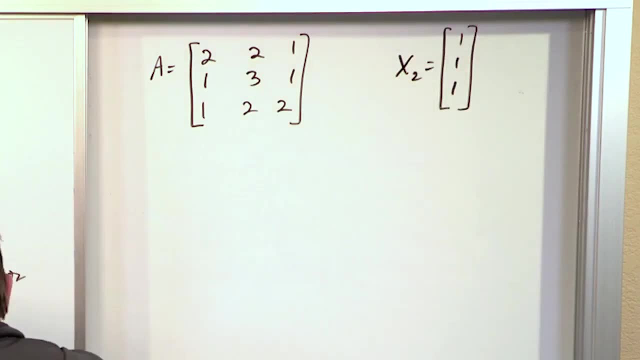 1, 1, 3, 1, 1, 2, 2.. And the potential eigenvector that we're testing is 1, 1, 1.. Okay, How do we figure that out? We run it through the eigenvalue problem. AX is lambda, X, All right. 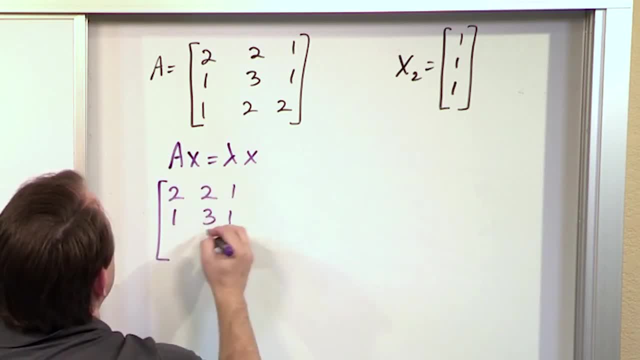 So the matrix we have is 2, 2.. 2, 1, 1,, 3,, 4, 5.. 1, 1, 3, 6, 7,, 7,, 8,, 9,, 10,, 11,, 11,, 12,, 13,, 14,, 15,, 16,, 11,, 12,, 13,, 40,. 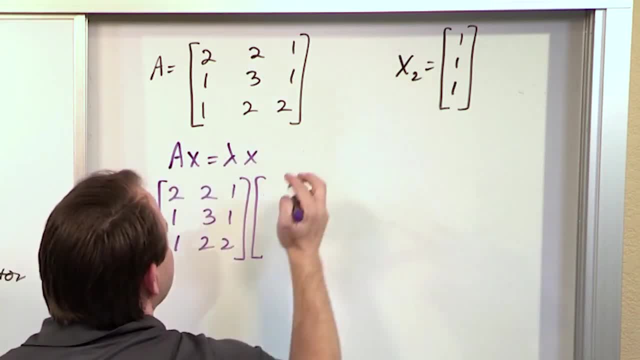 14, 14,, 15, 16.. And what we get.2, 1, 1, 3, 1, 1, 2, 2,. we're testing it by multiplying it by the potential eigenvector, And what do we get? Well, we're going to have 2 plus. 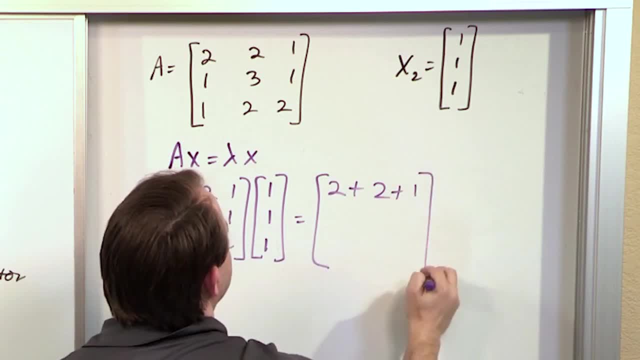 2 plus 1,- pretty easy to multiply. when you do this, It's going to be 1,, 3,, 1.. And then this across and down is 1,, 2,, 2.. And so, at the end of the day, I'm going to have 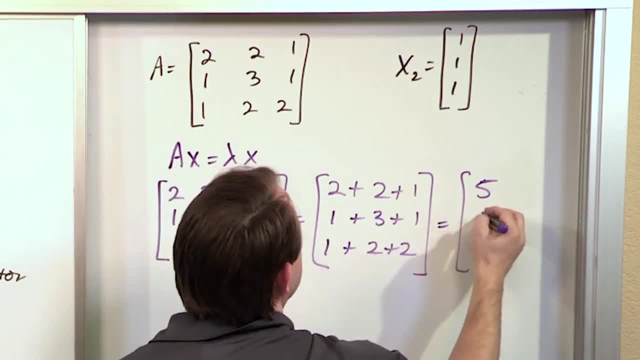 5, and then I'm going to have 5, 6, and then I'm going to have 2, 1, 1, 3, 1, 3, 1,이었 5,, and then I'm going to have 5, 6.. No 5.. This is going to be 5 as well, And then I'm going to have